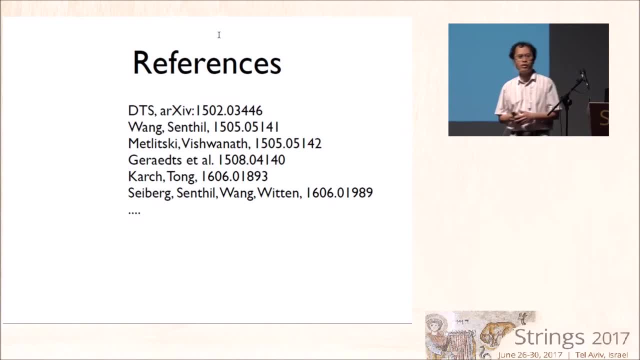 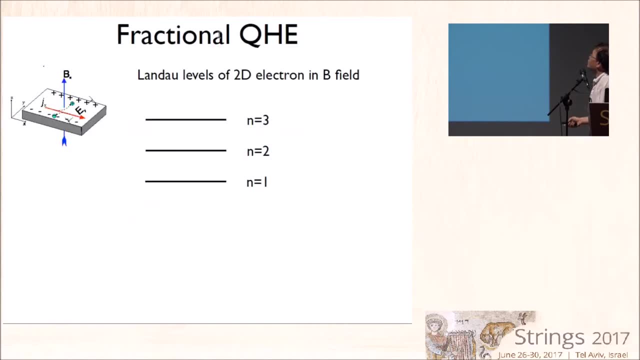 make it very clear that the physics of the quantum hole effects is tightly connected to the few theoretical dualities. So let us consider the two-dimensional system of electrons moving in a plane and in an external magnetic field. We know from 1930 that the spectrum of a particle moving in two dimensions in a magnetic field is organized in Landau levels. 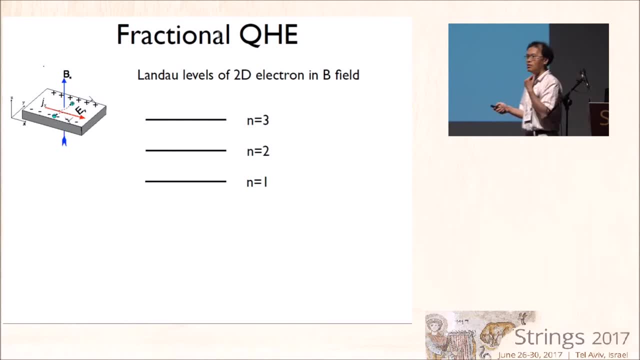 The Landau levels are discrete because the classical motion of the electron is periodic. Now suppose we have a large number of electrons, but the number of electrons is smaller than the degeneracy of the lowest level Landau level. Then we have a problem of finding a way to put these electrons on. 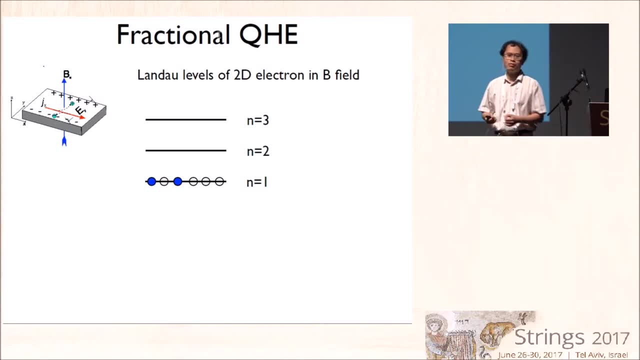 the lowest Landau level so that the energy is minimized, Ignoring the interaction. of course, we cannot solve this problem. So let me define a quantity called the filling fraction, which is a ratio of the number of electrons over the degeneracy of the lowest Landau levels. In this picture, nu would be: 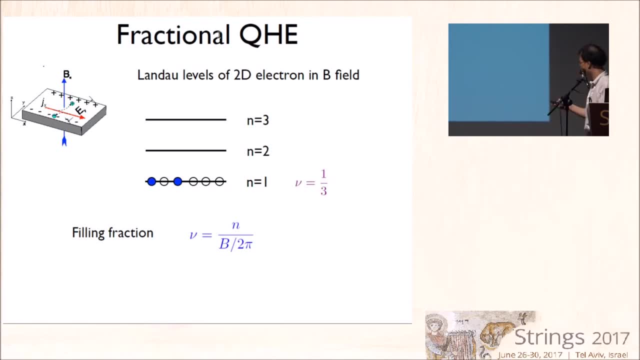 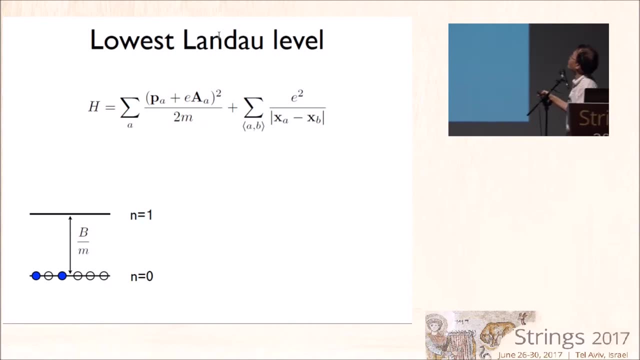 equal to 2 divided by 6, which is 1 third. The problem can be formulated like this: We have a Hamiltonian of n particles in an external magnetic field with some interaction- Let's choose here Coulomb interaction- And we want to find 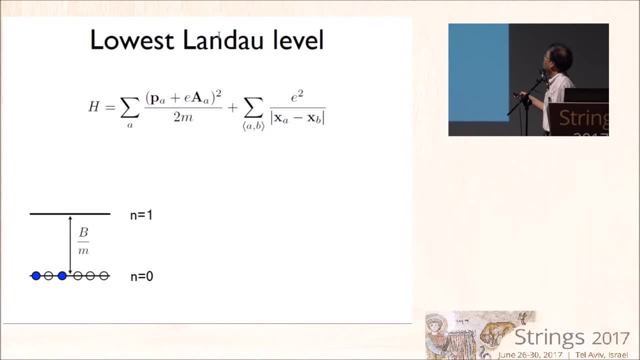 the ground state In the limit- let's take the theoretical limit- m goes to 0. Then the distance between the Landau levels becomes infinite. That means that we can ignore all the Landau level beside the lowest one. On the lowest Landau level, since the number of electron is less. 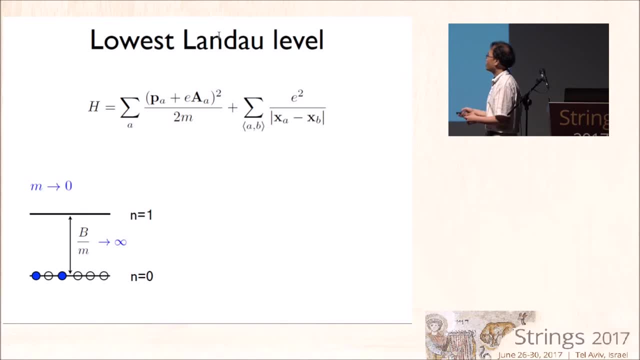 than the number of state available. there is a exponential degeneracy of state. if there wasn't the interaction, that would should leave the degeneracy, And so the problem can be formulated as trying to diagonalize the Hamiltonian, which is the Landau, lowest Landau level. projection of the 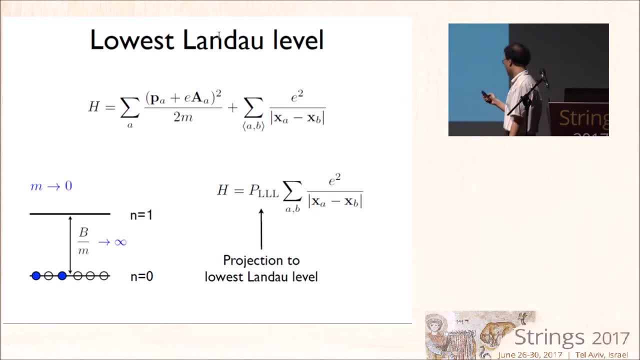 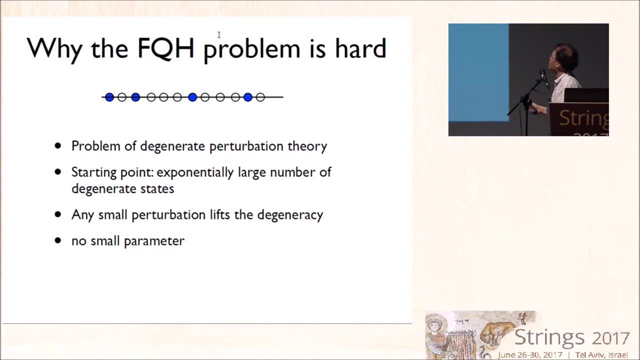 energy between the electrons. There is no small parameter that this fact makes the problem very hard. This is a problem with degenerate perturbation theory, with a starting point of an exponentially large number of degenerate state. What we are interested in is how a small perturbation leaves the degeneracy. So it seems that the 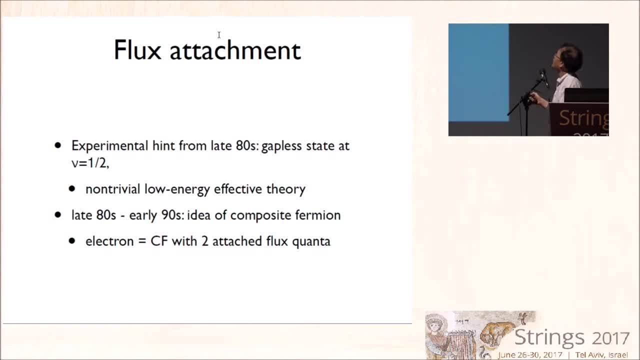 problem is very hard, but since late 1980s there is an experimental hint on the direction we should be thinking of in order to solve the problem, And the hint is that there is a gapless state at filling factor of half If the lowest Landau level is half filled. 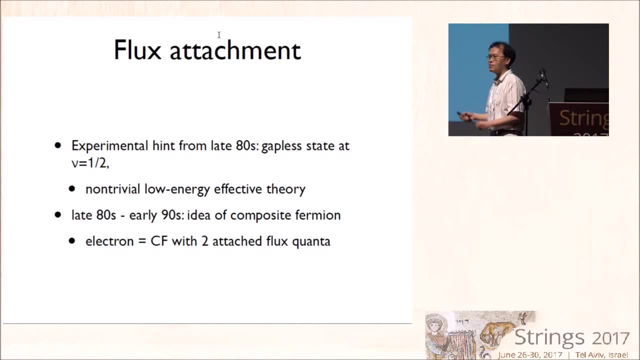 it seems that the system has non-trivial low energy degrees of freedom, hinting to a very non-trivial physics, And that led in the late 90s, late 80s, early 90s, to the idea of the composite Simmons. 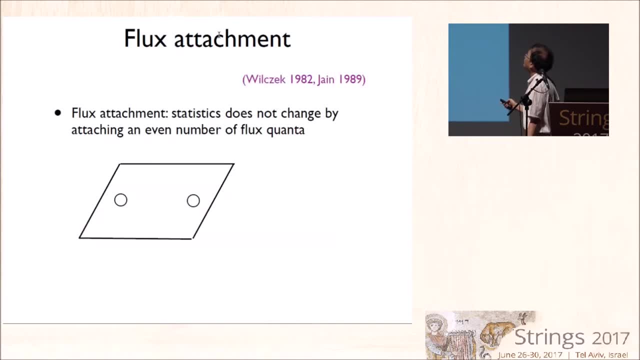 which I would like describe So here. the idea has the origin in the idea of flux attachment. The statistics of a particle does not change if we attach to a particle an even number of flux quoanta. So in picture, if we have two, 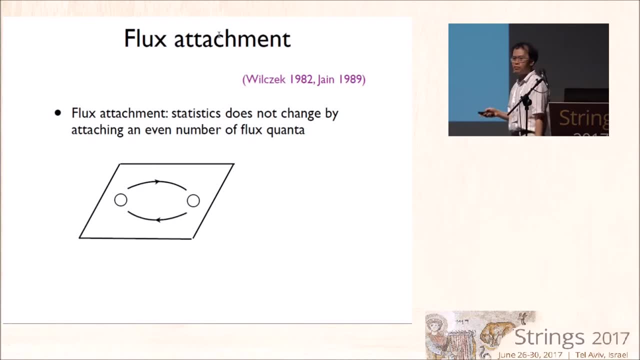 commented on. if we achieved them, will get them factor of minus one in the wave function. If now we attach to each of the fermions two magnetic flux quanta, then we get additional Aronoff-Bohm phase when we exchange the two. 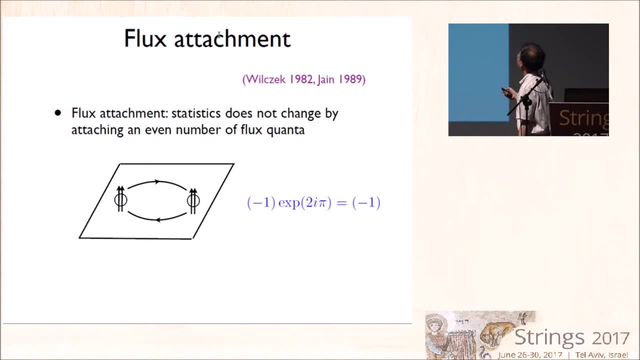 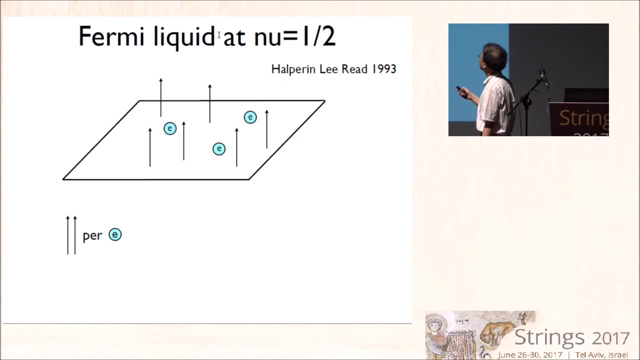 particles, but that phase is one in the case of an even number of flux quanta, and so the two particles are still fermions. This picture is formalized into a. so let me first explain why that leads to an understanding of the gapless nature of the new equal one-half. 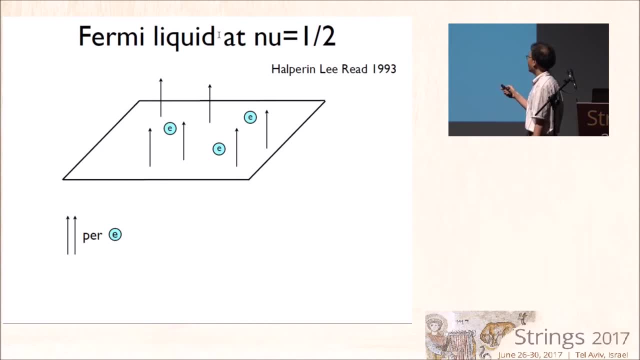 state. Suppose I have half as many electrons as the number of flux quanta going through the sample, and let me assume that I can represent this electron as another type of particle that we call composite fermion, plus two magnetic flux quanta. 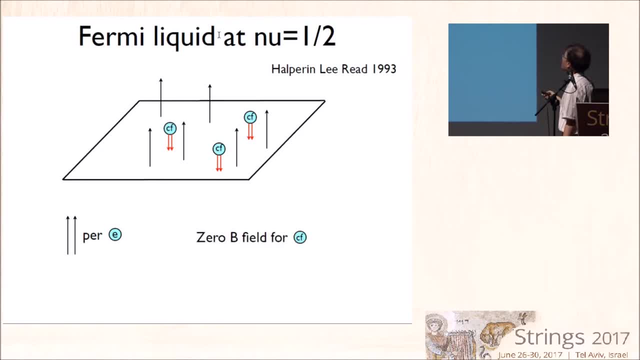 Then if one does a mean field approximation, we see that the new type of particle fuels a net zero magnetic field, a net average magnetic field being zero, And that means this particle would form a lambda Fermi liquid and the excitation 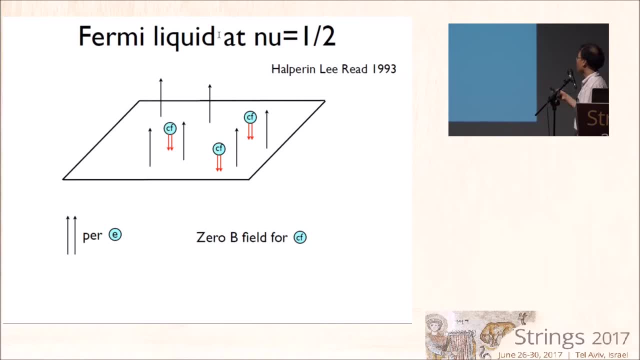 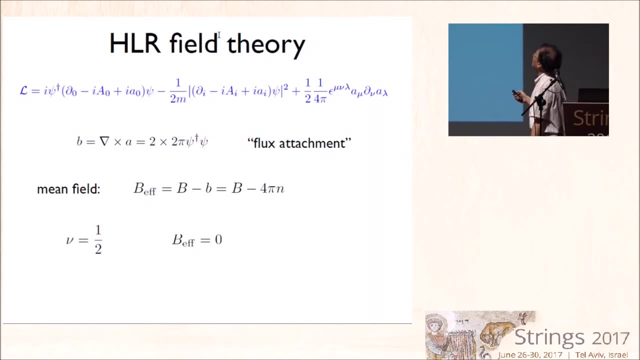 the low energy excitation will be gapless excitation near the Fermi surface. This leads to the formulation of the HLR field theory. Basically, it is a mathematical rewriting of the idea that has been presented in the previous slide. We have in this. 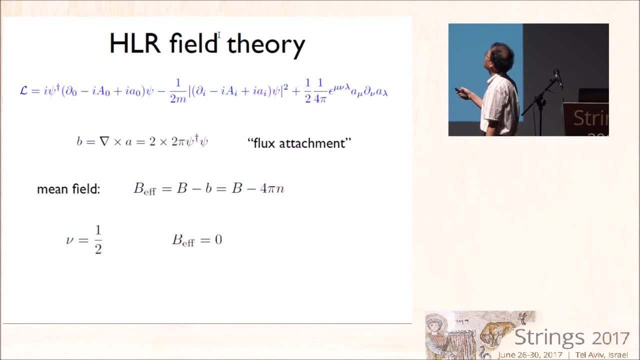 theory, a field, psi, which is a composite fermion which couples to the external electromagnetic field A and an internal field, A0, that has a Chern-Simons kinetic term And one of the equations of motion that we have we obtain by differentiating the action. 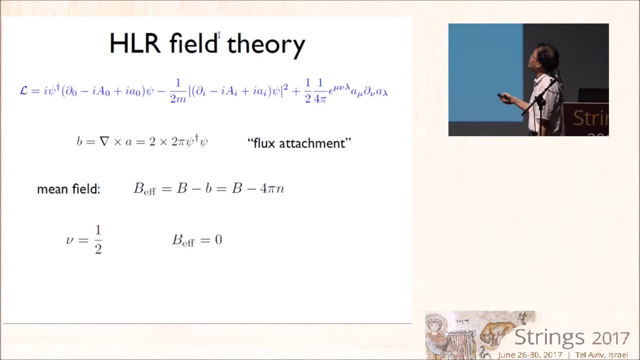 with respect to A0, tied to magnetic field B with the density of this fermion. Basically, each fermion leads to a delta functional magnetic field, just as we draw in the previous transparencies In the mean field. approximation then, 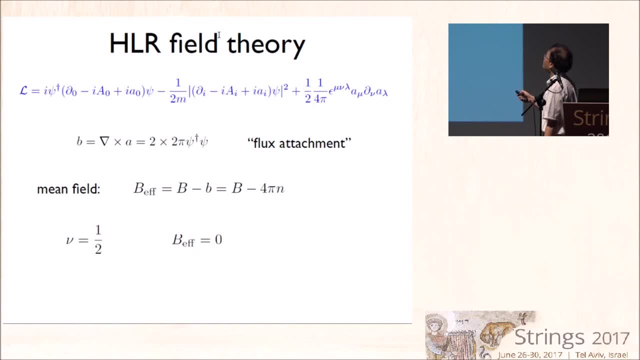 the effective magnetic field felt by this psi field is big B minus small b, which is B minus 4 pi times the density, The density of the fermion, and at half feeling the effective magnetic field is equal to zero. This theory implies that we understand. 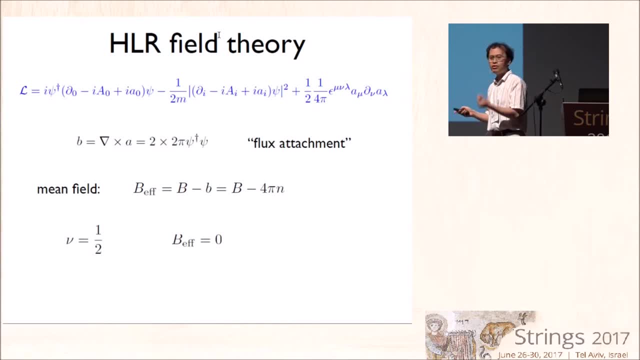 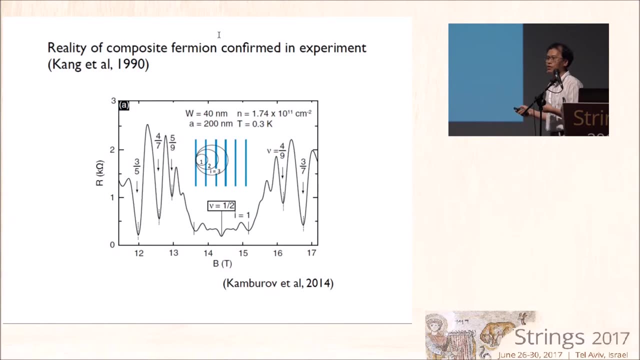 the nature of the gapless excitation near nu equal 1 half And there is actually experimental evidence that this is qualitatively the correct picture. So here is an experiment from 1990s in the newer version of the experiment from 1990s. 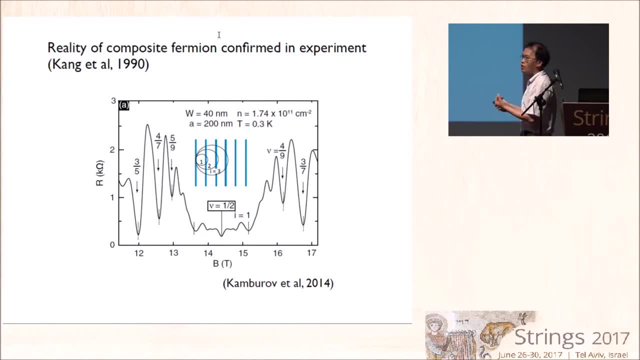 when one basically looked for semi-classical trajectory of this quasi-particle. An electron in a magnetic field moves in circular orbit, but this quasi-particle feels a much smaller magnetic field and you can tune that magnetic field to give this particle almost a straight orbit. 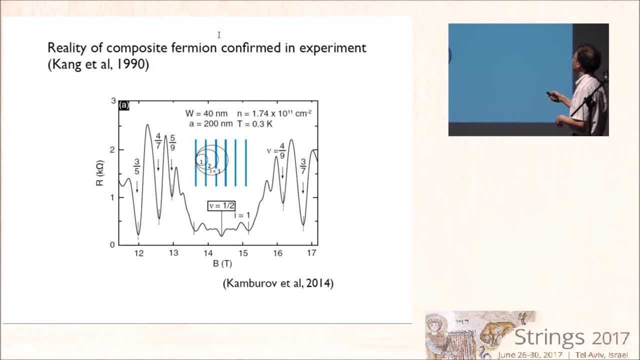 So here, if you tune the feeling factor to nu equal 1 half, this particle will shoot in a straight line and in this, if you go around nu equal 1 half, you can find a very large semi-classical orbit of this particle. 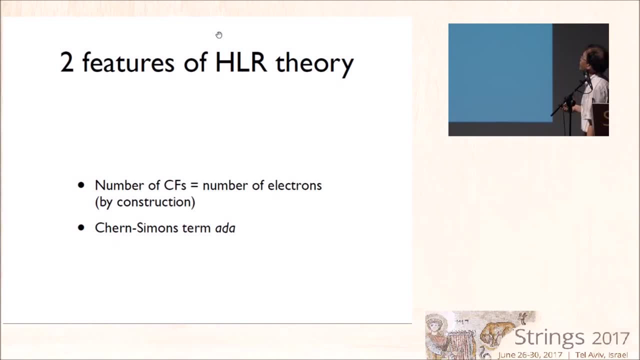 Two main features of the HLR theories that I want to emphasize here is that, first, the number of the composite fermion is equal to the number of electrons. This is by construction, by the philosophy of flux attachment, And tied to that is the Chern-Simons. 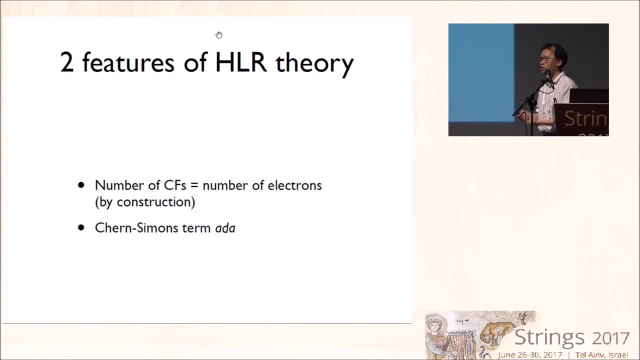 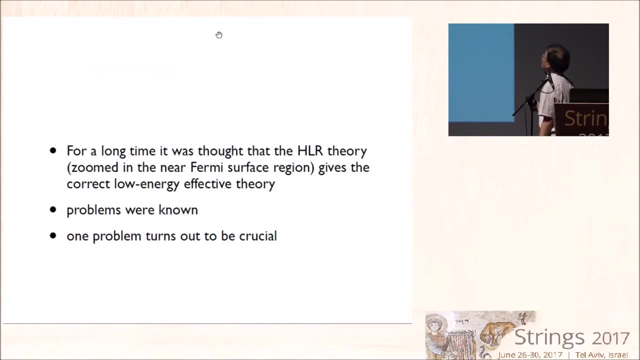 term ADA. that leads to the uh relationship between the magnetic flux and the number of particles. For a long time it was thought that the HLR theory is the correct theory of the low energy degrees of freedom of the half-field and down level. 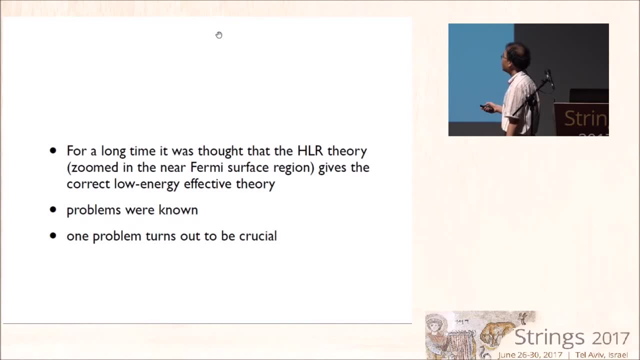 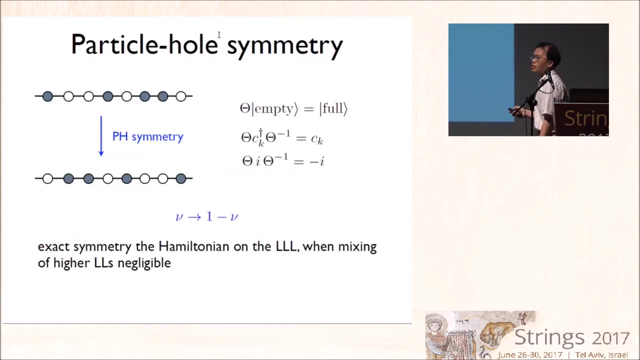 Some problems in this theory were known and some were thought to be serious, but one of the problems that was mostly neglected turned out to be crucial, And that is the problem of particle-hole symmetry. Imagine that we are dealing with a single Landau level. That means 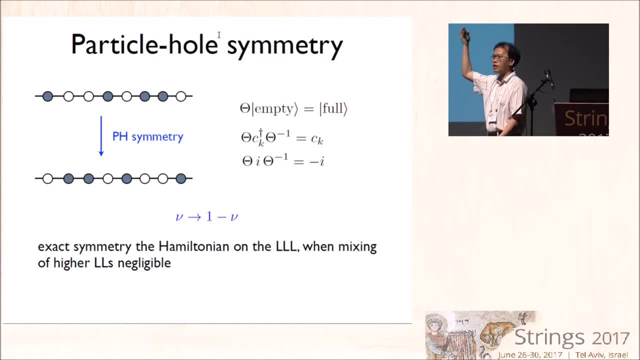 we are, the distance in energy to the next Landau level is very large. Then we can define an operation that changed a state in the Hilbert space on the lowest Landau level to another state in the following way: Any state on the lowest 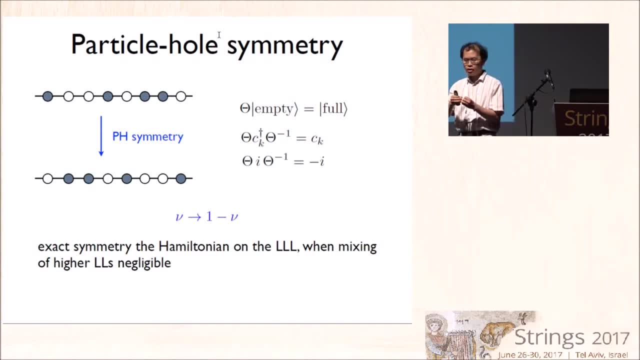 Landau level can be extended. uh can be presented as the linear combination of state in the uh occupation number basis. We occupied some orbital and left some state unoccupied. The particle-hole conjugation map such a state in a mirror state in which the unoccupied 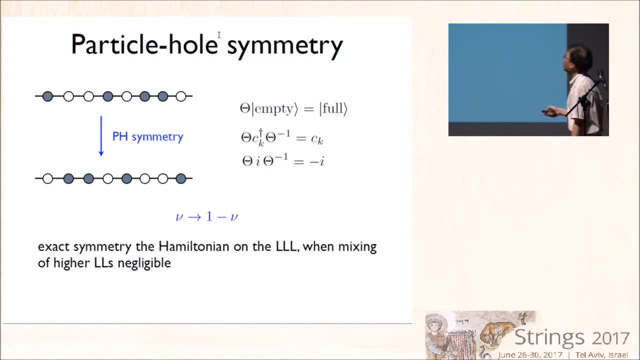 orbital becomes occupied and vice versa, And one can define formally this operation. It flips the roles of creation-annihilation operator. It's also a natural, most conveniently defined as the anti-unitary transformation. The important thing is that it makes new map, new into. 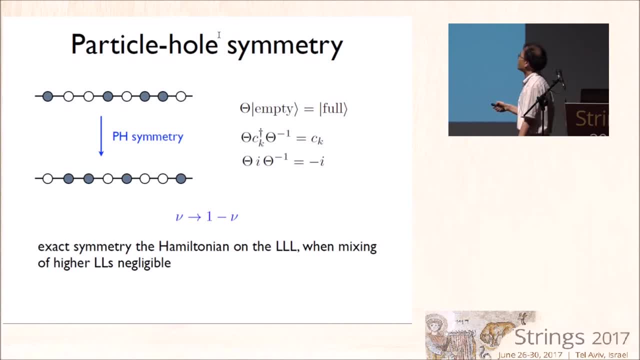 one minus new, which means that a half-field state becomes a half-field state, Or in other words, a half-field Landau level is at the same time a half-empty Landau level. One can define such a transformation And one can show. 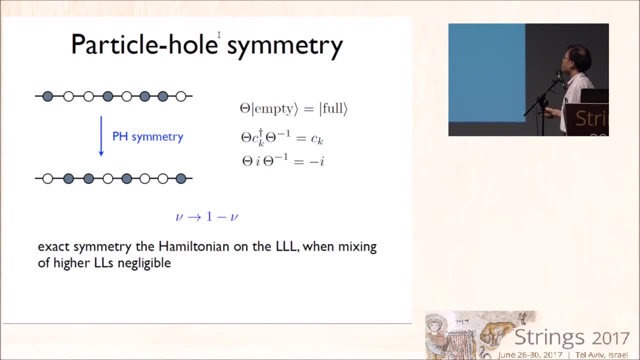 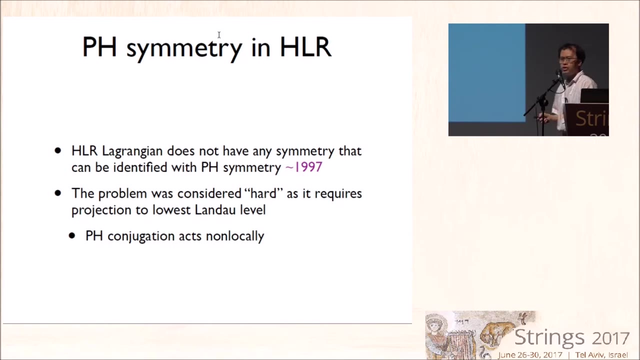 that this symmetry, this pH conjugation, is an exact symmetry of the Hamiltonian if the interaction between particles is pairwise. However, the HLR Lagrangian, which we thought was a low-energy description of the dynamics of the half-field Landau level, doesn't. 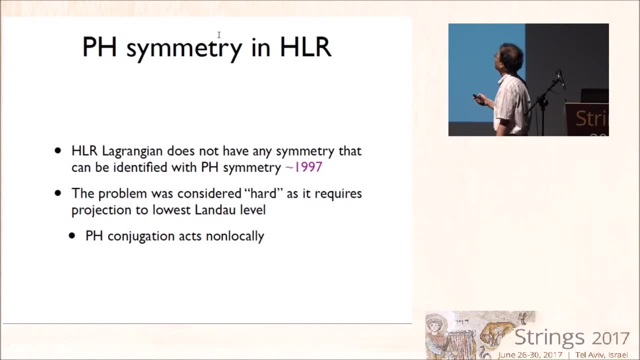 have any symmetry that can be identified with the particle-hole symmetry. This problem has been known probably since 1997. at least It was considered as a hard problem in the hierarchy of problems in quantum-hole physics because it required projection to the lowest Landau level, which makes 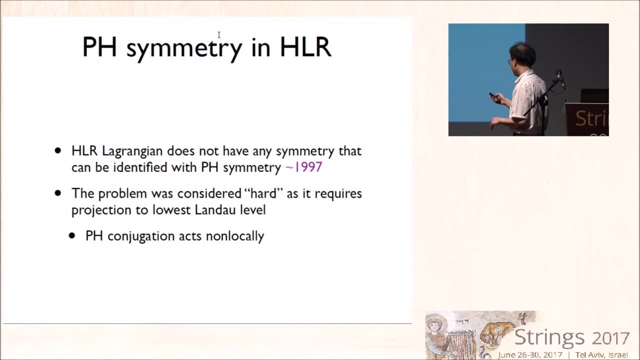 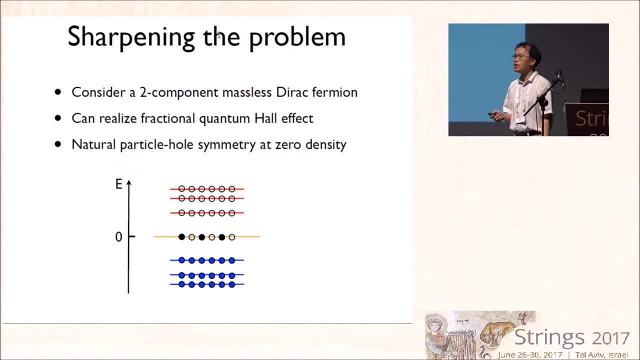 everything non-local. So a progress is made by sharpening this problem, by considering a quantum-hole effect in a slightly different context but essentially with the same physics. Consider two components: mass-less Dirac-Fermion, So Dirac-Fermion in 2 plus 1 dimension. 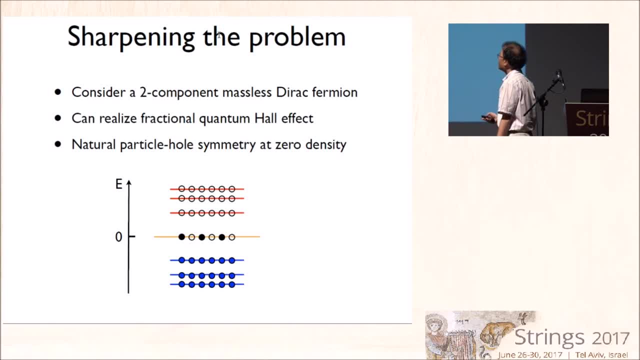 in a magnetic field, Then we can solve the Dirac equation and obtain the spectrum, the Landau level, which now would stretch from minus infinity to plus infinity. The Dirac-C becomes negative energy levels. But the main thing is that there is 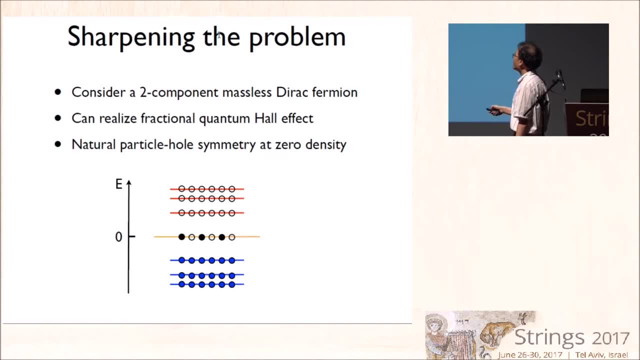 a symmetry, E to minus E in the spectrum, and there is one exact energy level with zero energy. Now, if we have zero chemical potential, that means that we have to decide which state in the zero level of the Hamiltonian to fill which one. 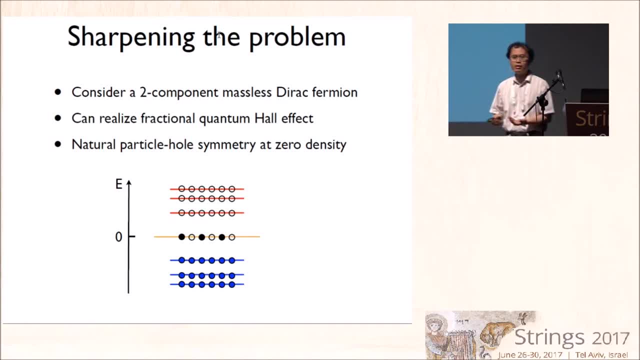 is left empty, And this is now exactly the same fractional quantum-hole problem as we have in the non-relativistic case, Except here that we have more symmetry. The relativistic symmetry of the spectrum of the Dirac-Hamiltonian implies that we have a natural 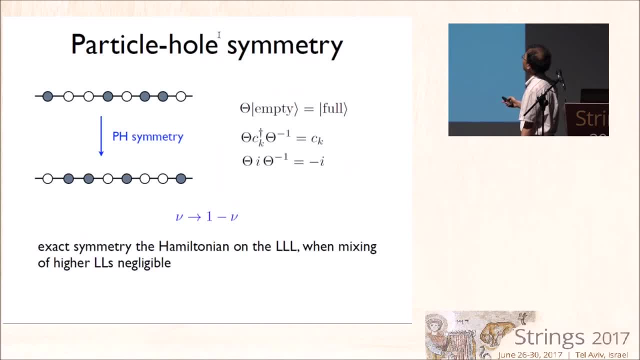 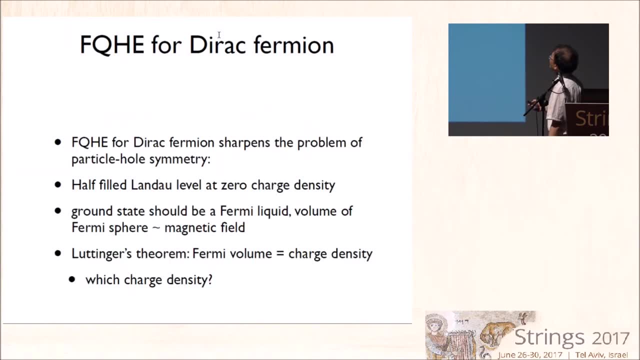 particle-hole symmetry that does not require projection to the lowest Landau level, And so the fractional quantum-hole effect for the Dirac-Fermion, which should exist because it's basically based on the same principle of the degeneracy of the Landau level as the usual fractional 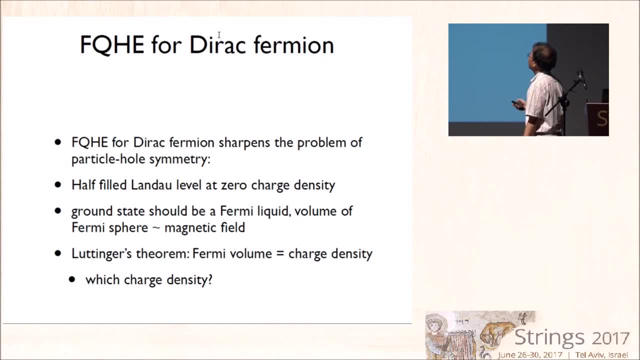 quantum-hole effect. it sharpens the problem of particle-hole symmetry There is now. we don't even need to project to the lowest Landau level to have particle-hole symmetry. The half-field Landau level appears at zero charge density. Now that implies another 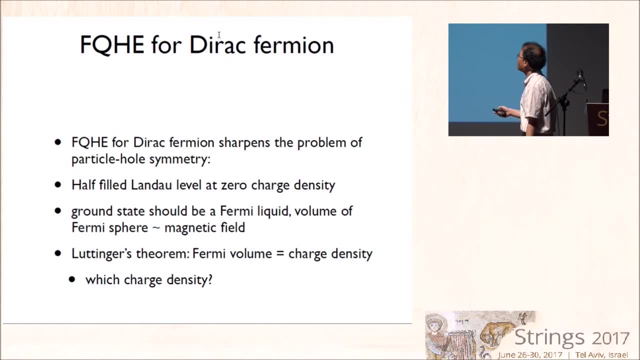 problem for the HLR philosophy. The problem is the following: We know that a half-field Landau level from experiment that it has. it is a Fermi liquid. A Fermi liquid with a Fermi rate with a volume of the Fermi sphere being 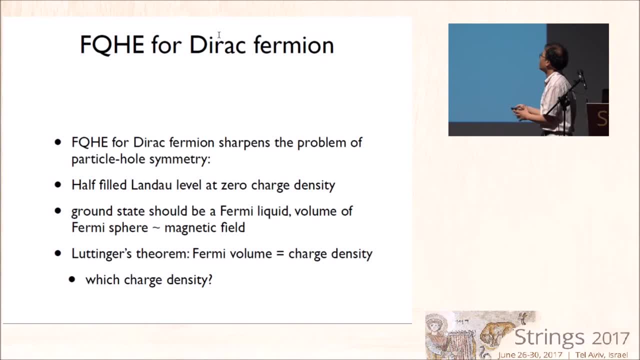 equal to the number of particles on the lowest Landau level, which is proportional to the magnetic field. On the other hand, we know from many body physics that there is an exact theorem, called the Lattinger theorem, proven for very large classes of. 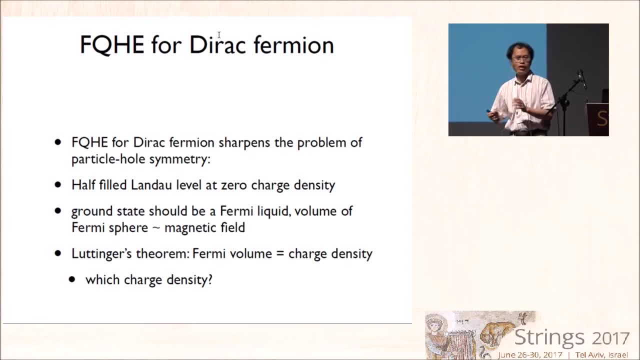 Fermi liquids and believed to be valid also for some non-Fermi liquids, is that the Fermi volume, the volume enclosed by a surface where the fermionic excitation is massless, is equal to the density of a conserved charge. But now, in the 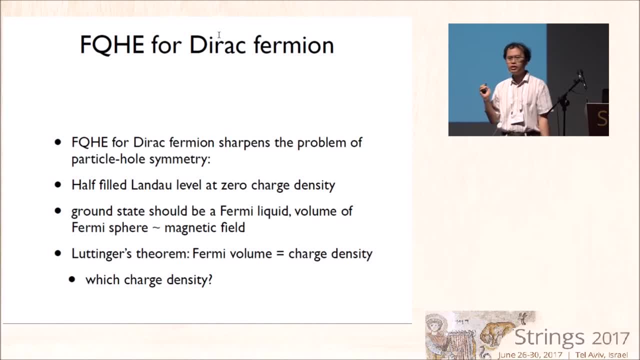 relativistic problem. the conserved charge density is zero, because we put the chemical potential exactly going through the zero energy level. And so if that charge density is the density of the electron, then it is zero. Then we have a problem with Lattinger theorem. So there, 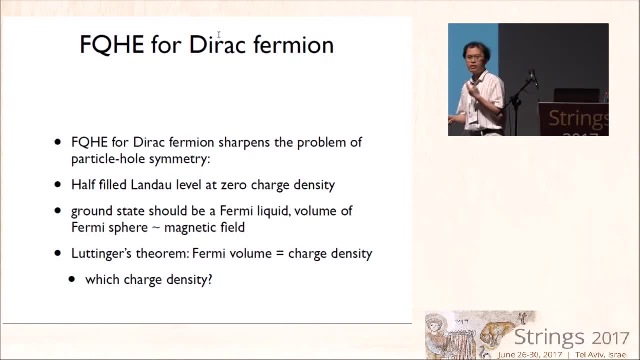 is another ah puzzle that we get by considering fractional quantum Hall effect in the relativistic case. somehow this relativistic system puff up a Fermi surface, but when we turn on a magnetic field we don't. we don't have to turn on any chemical potential to pop up a Fermi surface. a magnetic field itself create a. 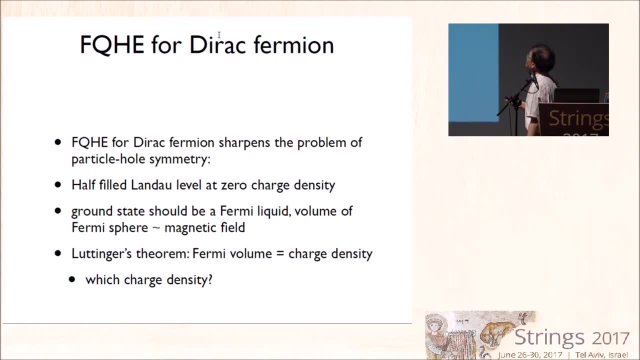 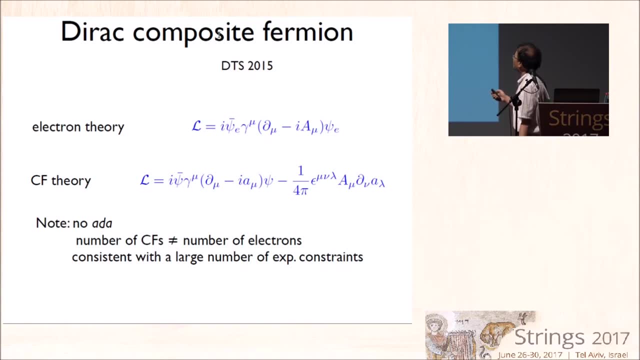 Fermi surface. so this led, after some try and error, to proposal of a new, presumably more correct theory of the low energy degrees of freedom of the half-fuel and our level if we have some electron coupled to external electromagnetic fields. you know background of a magnetic field with some 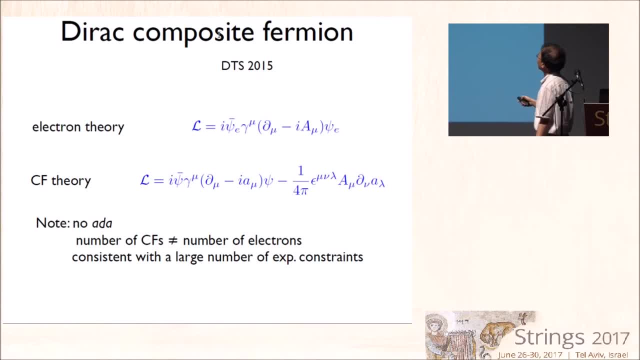 interaction between the electrons. the low energy theory must have the form of direct fermions, two-component direct Fermion coupled to a dynamic, to a dynamical gauge field which has some churn Simons type of thank you of mixing with the external field. there are two things that distinguishes this theory. 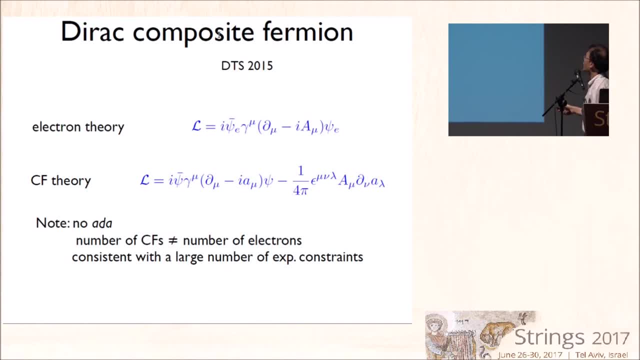 from the HLR theory. the number of the composite fermion is now not tied to the number of of electron. in fact, these composite fermions now are not tied to the number of electron. in fact, these composite fermions now are are not directly coupled to the external electromagnetic field. 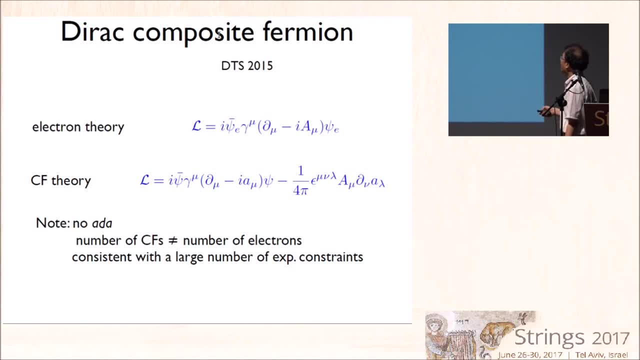 They are electrically neutral And this theory turned out to be consistent. and there is no Chen-Simons ADA term. It turned out that this theory is consistent with a large number of experimental constraints that I will not mention. So one thing that this type of Lagrangian implements. 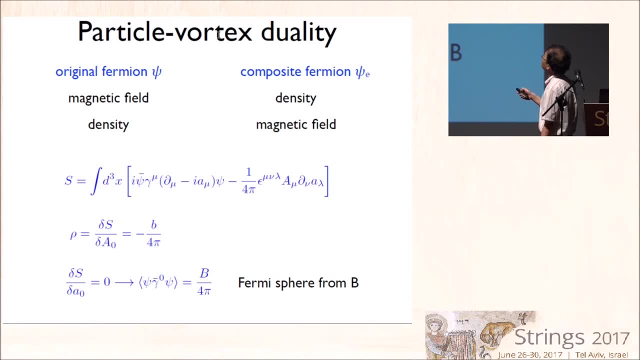 is exchange between the notion of the magnetic field and the notion of density. What was in the term of the original fermion was the density becomes the magnetic field felt by the composite fermion, and vice versa. the external magnetic field is equal to the density of the electron. 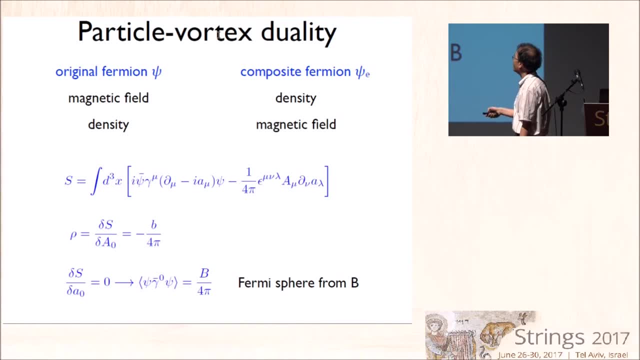 So, for example, if you differentiate this action with respect to A0, you find right away that there is a constraint between the density of the composite fermion this side with the magnetic field, which explains why, turning on the magnetic field, 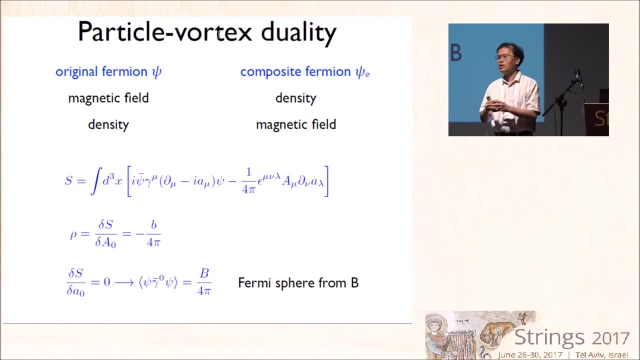 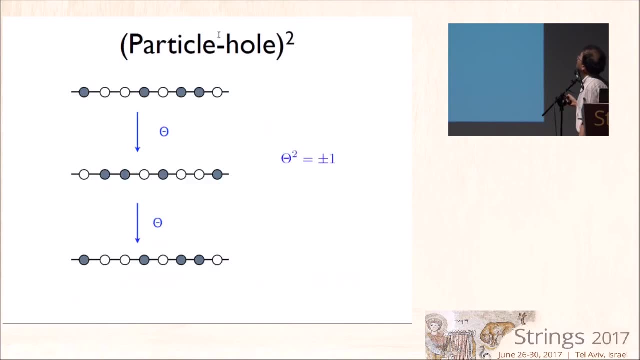 can create a Fermi surface without any chemical potential. So there is Looking backward. there is The fact that the composite fermion should be The Dirac fermion actually could have been figured out some time ago by just thinking about the physics. 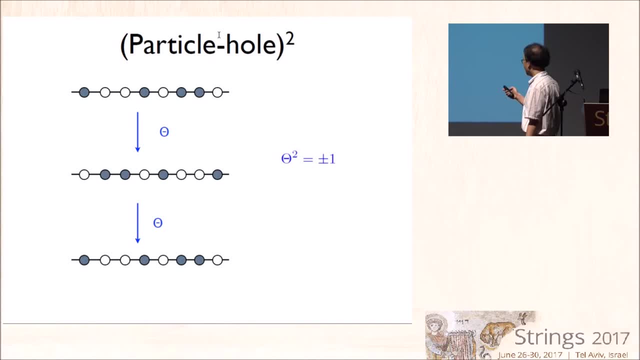 of the lowest Landau level. The important thing is that the particle-hole conjugation is an anti-unitary transformation and its square can be either plus one or minus one, And the case when it's minus one is non-trivial. So, on a single Landau level, 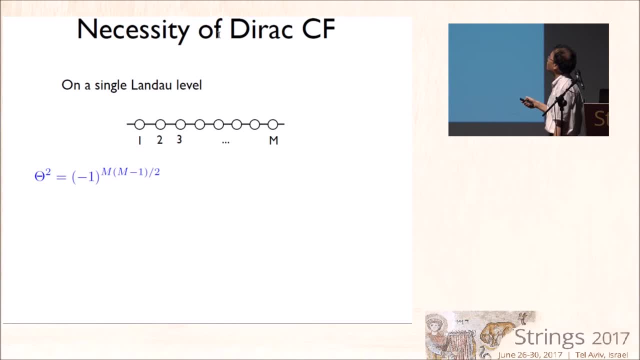 theta squared is equal to minus one to m. m minus one divided by two, m is the number of state on the lowest Landau level, And if m is even, then we can represent that as minus one to some number, And that number is naturally identified. 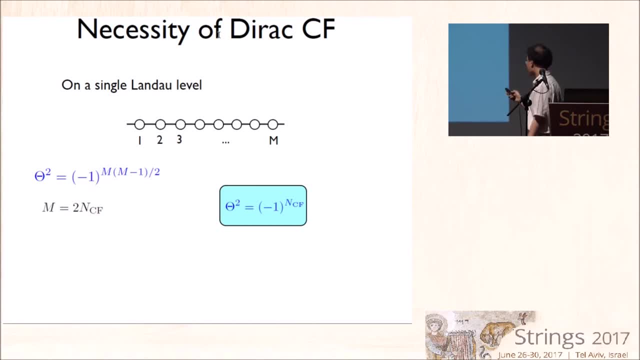 with the number of composite fermion. So if that identification requires that the number of composite fermion has to be half of the number of flux quanta and should not be equal to the number of flux quanta, then that number is equal to the number of electron s. 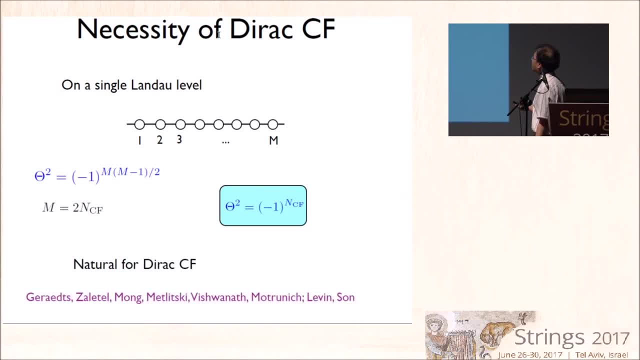 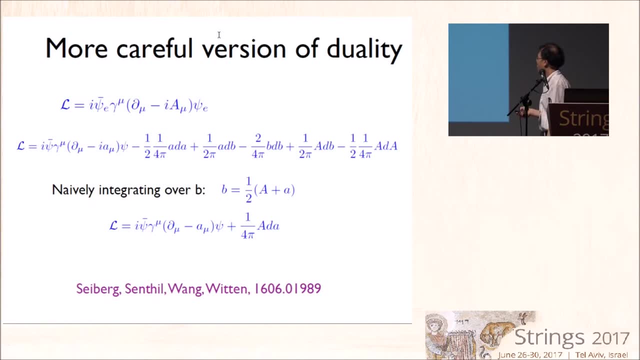 as the HLR theory will tell us. Okay, so the more careful version of this duality was found, pointed out. it was pointed out that the version of duality that I have just presented to you does not satisfy the matching of anomalies and Seiberg's. 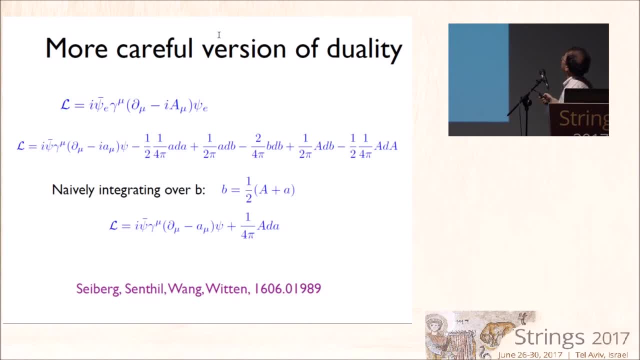 until Wang and Witten wrote down a more careful version of this duality. If one takes this Lagrangian and naively integrates over B, ignoring the fact that the flux of B might be not an integer, we find the naive duality that I have presented to you before. 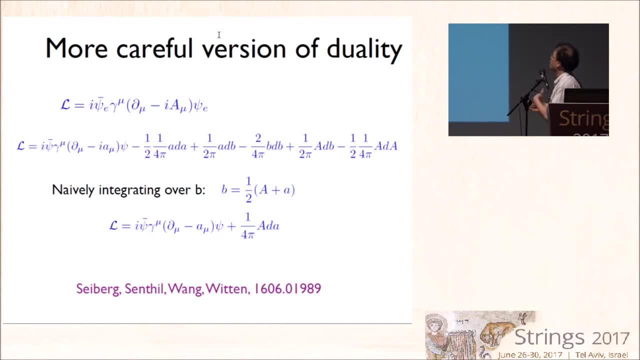 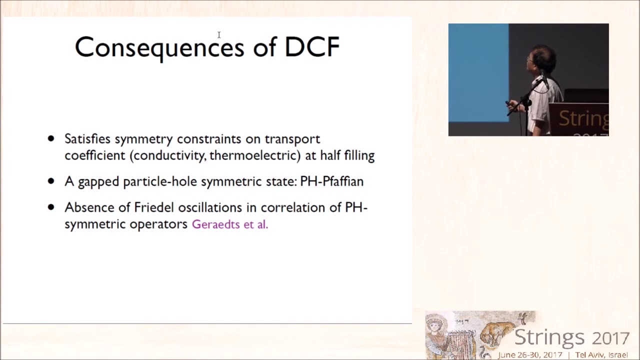 But all what I have told you about the physics of the Fermi surface would remain the same in this theory. So there are some consequences of the Dirac composite fermion theory. First, it satisfies symmetry constraints on transport coefficients, the conductivity thermoelectric constant. 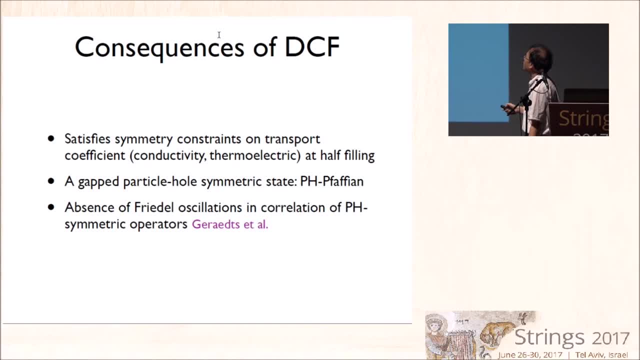 It implies a possible existence of a new gap particle-hole symmetric state that may be realizable in quantum-hole systems, called the pH-Pafian state, And it's predicts the absence of Frieder oscillation in correlation function of certain symmetric operators. 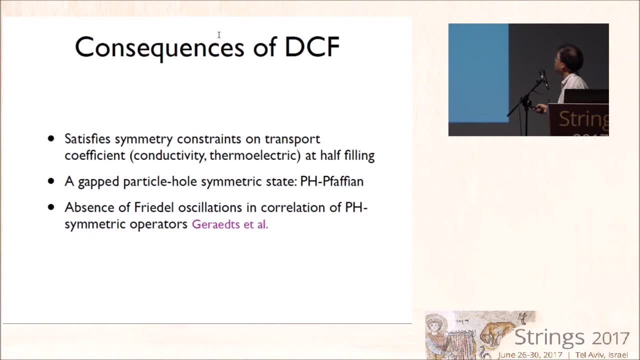 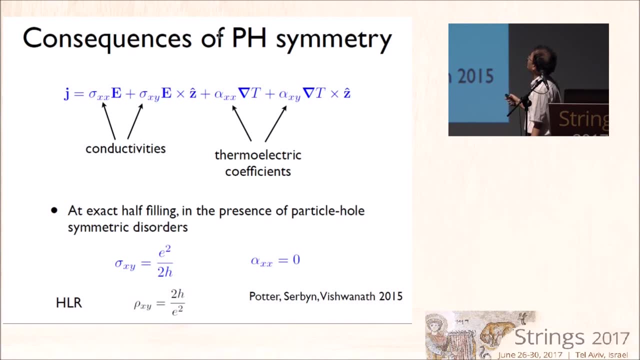 And this has been checked numerically. Let me go through a few of them. One can define the conductivity and the so-called thermoelectric constant by looking at the current in external electric field and gradient of temperature- An exact half-fueling if the particle-hole symmetry is exact. 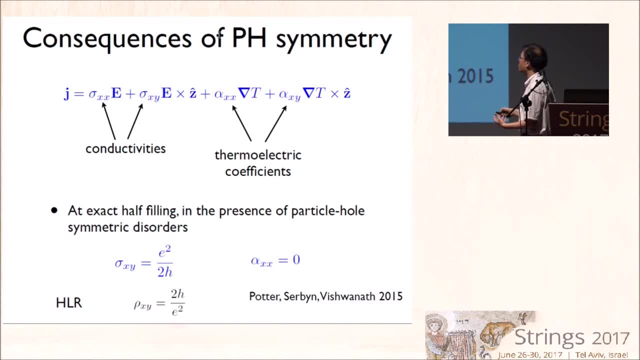 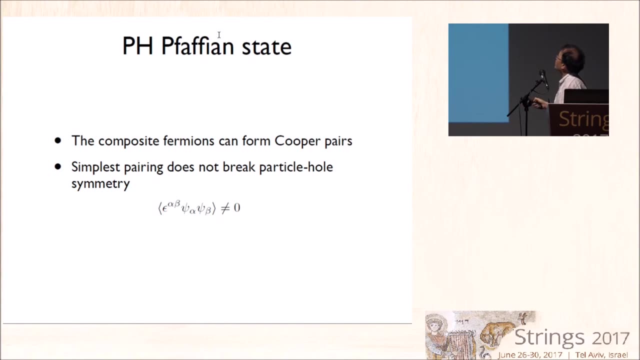 then sigma-xy. the hole conductivity has to be exactly one half of the quantum and one of the thermoelectric constant has to be zero. So this is a consequence of particle-hole symmetry. Another consequence is that the composite fermions conform a Cooper pair. 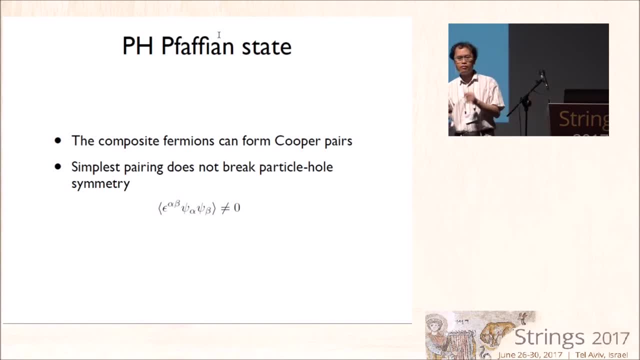 If one imagines some possibility of tuning the interaction between the fermions, the simplest pairing does not break particle-hole symmetry. This is the pairing that leads to a state that is non-Abelian state, which is different from the Phafian and the anti-Phafian states. 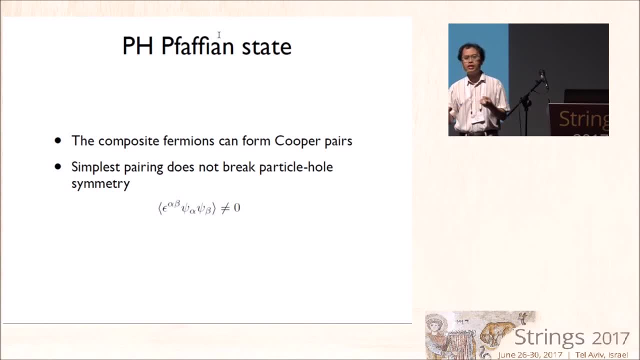 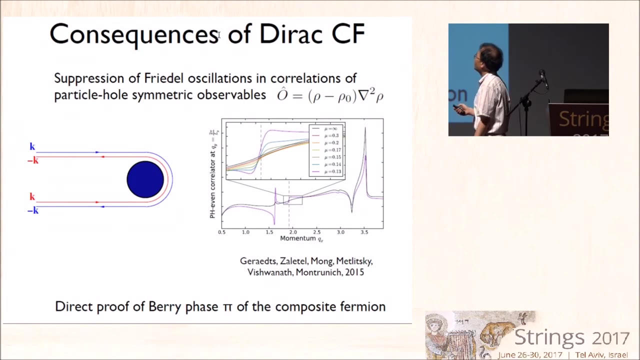 which are the two gap states that has been known before in the context of nu, equals 5 half, that is, half-fuel- and equals 1 Landau level. And the most non-trivial question and one of the consequences of this symmetry: 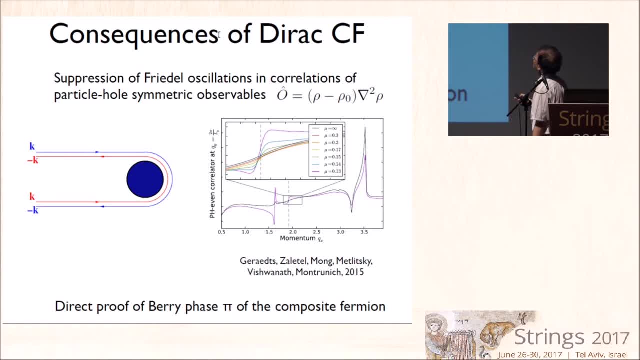 and the one that has been checked numerically is the suppression of Friedel oscillation in correlation of particle-hole symmetric observables. Suppose I have two operators. I take an operator O which does not map to itself under particle-hole symmetry. 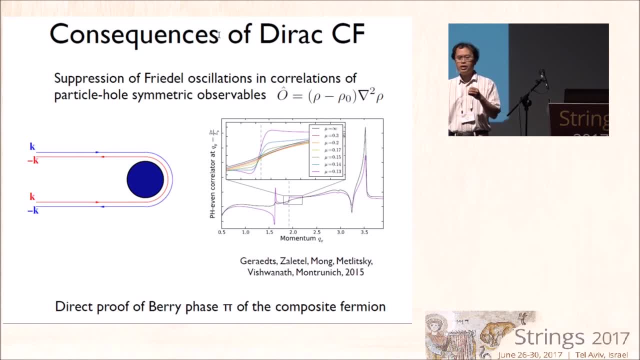 and compute the correlation function in momentum space, Usually in condensed matter physics, if we have a Fermi surface, this correlation function has a singularity when the momentum is equal twice the Fermi momentum. That's because we can create a particle-hole pair. 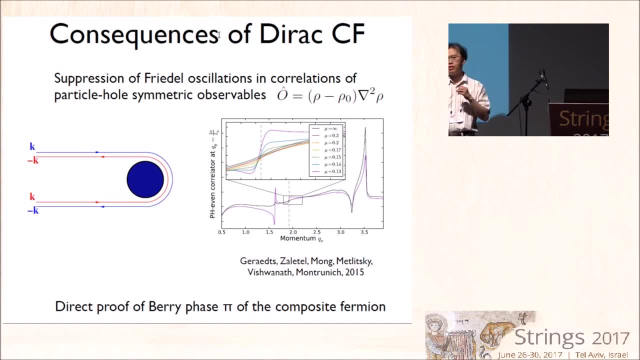 when the particle is near one pole on the Fermi surface and the hole is near the opposite pole of the Fermi surface, And the singularity of the phase space explains the singularity of this correlation function, and this is called Friedel oscillation. 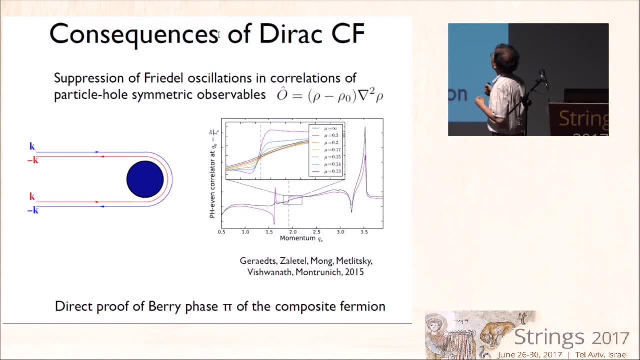 And it turns out that one can show this. the leading singularity disappears by symmetry reason if the operator maps to itself under particle-hole symmetry. And these people have simulated the Hartfield-Landau level and found that when we tuned the Hamiltonian to be particle-hole symmetric, 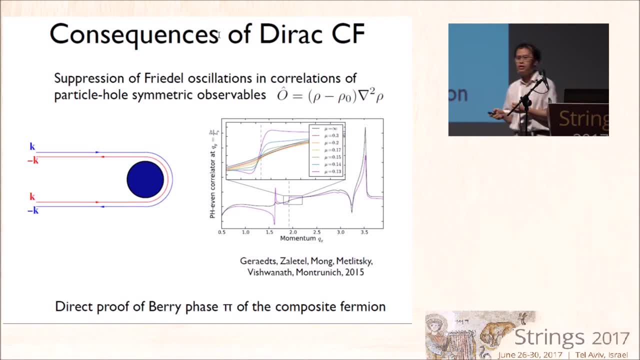 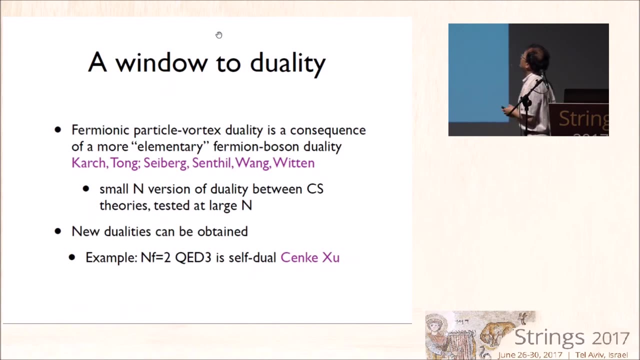 the Friedel oscillation disappeared, which cannot- I don't know any other explanation rather than the explanation based on the Dirac nature of the composite fermions. So the fermionic particle-vortex duality can be derived from a more elementary fermion-boson duality. 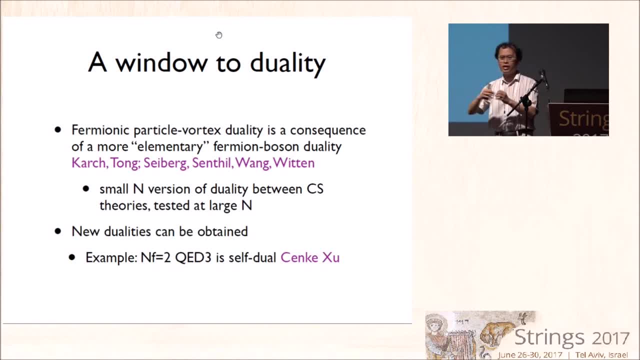 Taking a fermion-boson duality and applying it one more time after taking time reversals, one can derive the duality between the electron theory and the composite fermion theory. The elementary boson-fermion duality can be thought of as the small n. 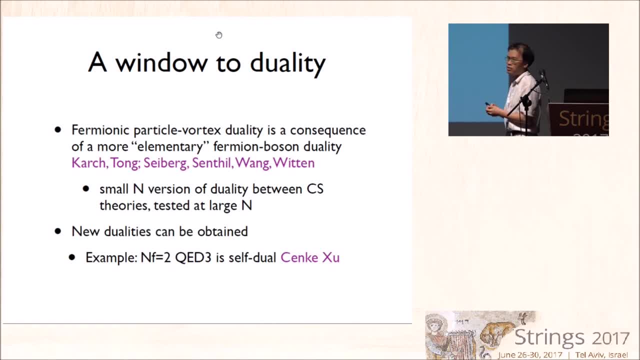 n equal 1, basically version of the duality one duality between Chern-Simons theory that has been tested at large n. But this is a really small n case. Using these dualities, new dualities can be obtained. in one example that: 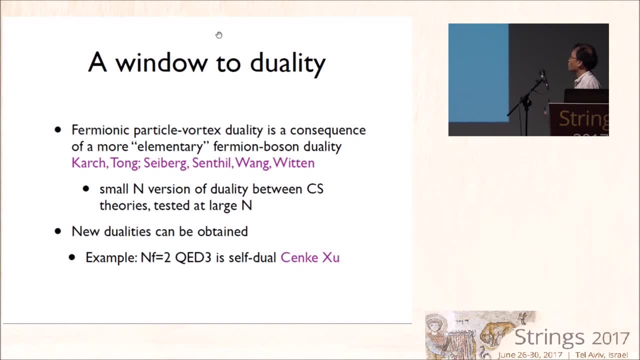 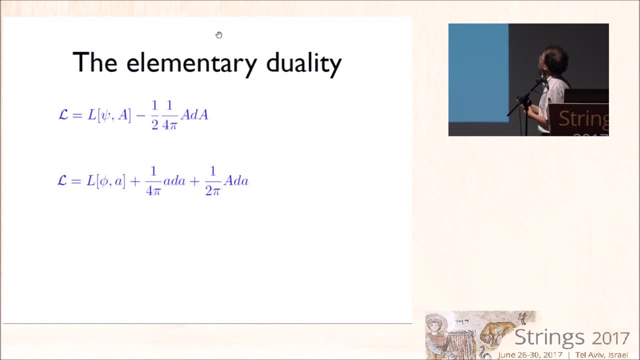 is also interesting is nf equal 2, QED in three dimensions can be shown to be self-dual, So the elementary duality looks like a map between a theory of a single fermion, two-component fermion with the scalar. 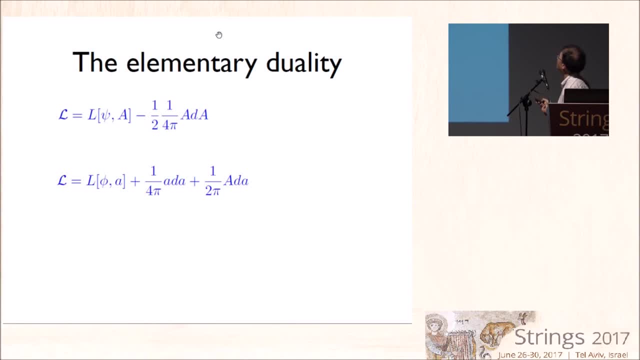 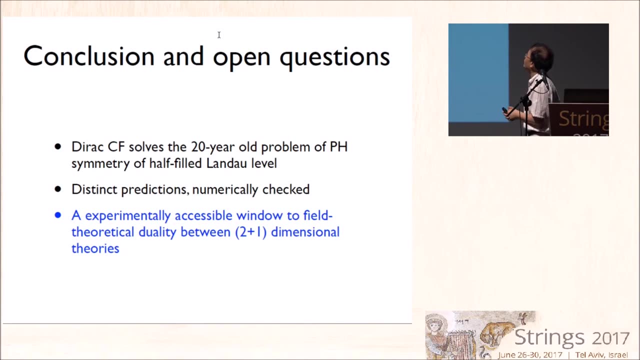 with the Chern-Simons interaction. So let me go to the conclusion. The Dirac composite fermion theory solved a 20-year-old problem of particle-hole symmetry of the half-field Landau level. It gives a new understanding of the low-energy dynamics. 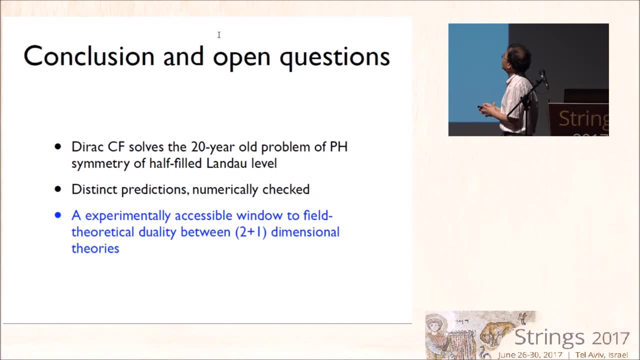 of the half-field Landau level, and it gives distinct predictions, some of which has been numerically checked, And what is interesting, for me at least, is that it is what can be. one can think about this quantum-hole system as experimentally accessible. 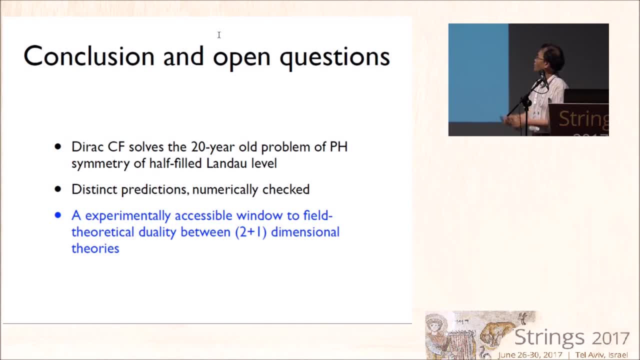 accessible windows to some small part of field-theoretic duality between two plus one dimensional theories. Thank you very much. Are there questions? Do I understand correctly that you are saying that the theory of Halperin et al is dual to the theory you have? 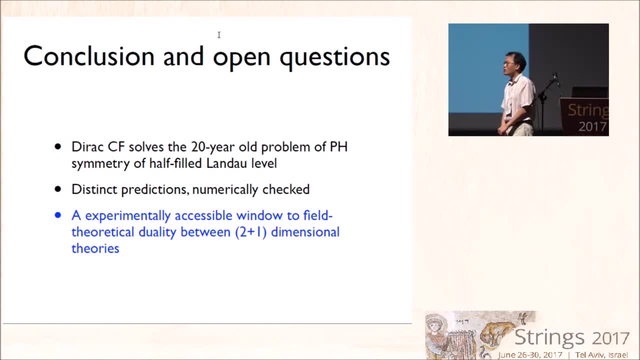 Is that the statement? There is a work by Halperin Stern Wang where they computed two physical quantities and they see that they satisfy. for these two quantities particle-hole symmetry is satisfied and they reproduce the result of the Dirac composite fermion theory. 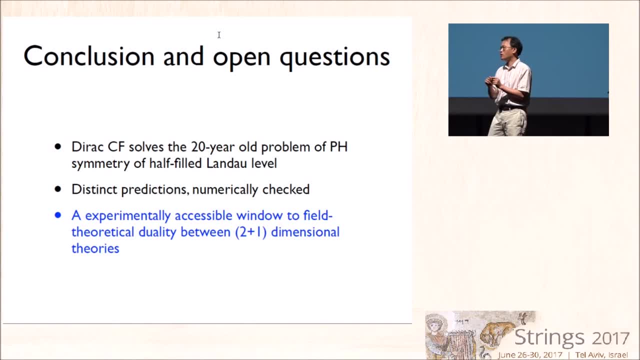 I believe this is a coincidence. There are, if one takes generic correlation function, like correlation function of two currents. doing the calculation, I did the calculation and the HLR theory gives results that are not particle-hole, symmetric and distinct from the Dirac theory. 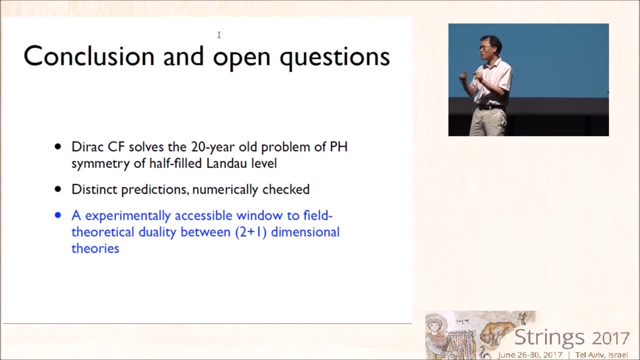 in most of the cases, These two cases are somehow very. these two quantities are really special. Oh, I see. So you have a theory which is different from their theory and I didn't understand the role of duality. So you had this theory. 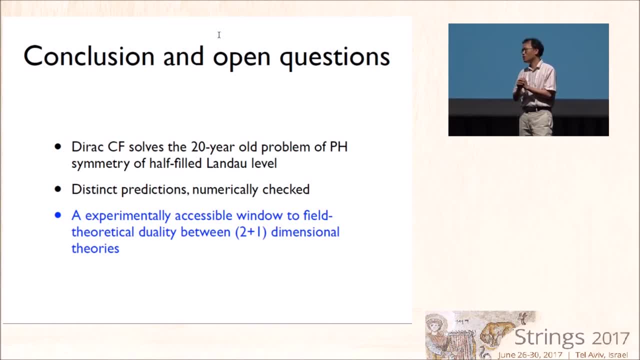 Why is duality playing a role? Well, it does provide at least philosophy that would replace the philosophy of flux attachment. The old picture of flux attachment is very attractive because it's really intuitive. You just take the electron and transform it somehow into a composite fermion. 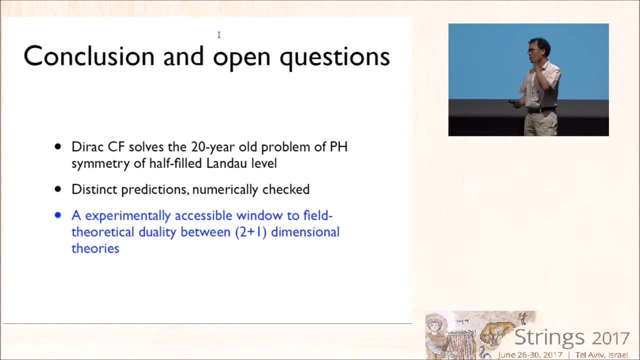 To me that sounds like a phenomenological rule, that. but it sounds more natural from field theory to say that you write down Lagrangians that are natural with terms and so on. So I'm not sure why we need to invoke flux attachment. 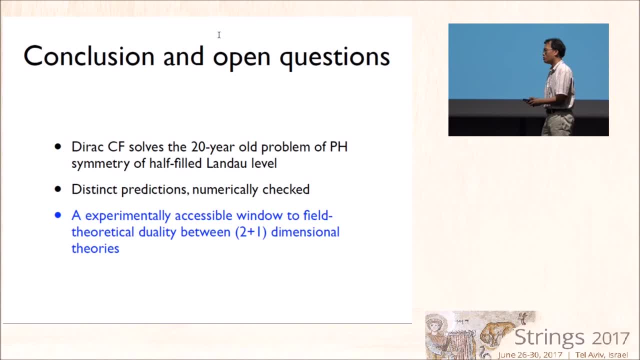 It sounds like it's a rule that gives the wrong answers for this problem. I'm sorry, I don't understand your question. So you ask: why the I need the direct, I need the duality, Why do you need flux attachment? 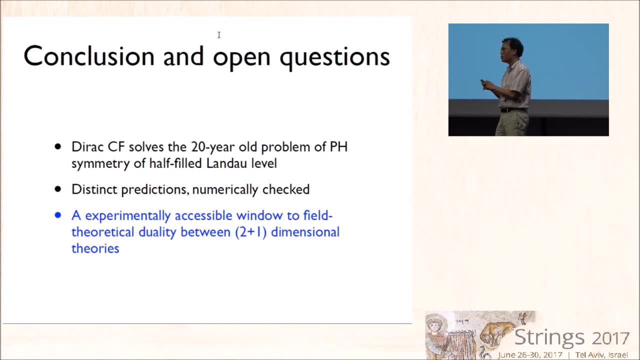 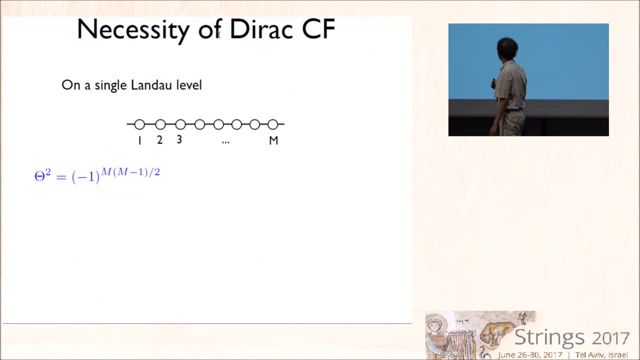 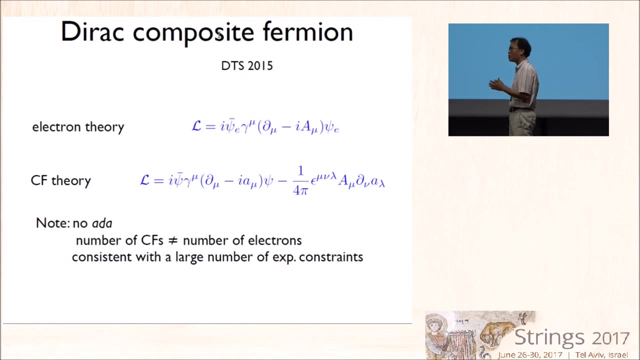 Why do you need this picture? Why don't you just simply write down Lagrangians with Chern-Simons terms, as you are doing? Well, that's basically what I did, That is, write down a theory that satisfies the symmetry. 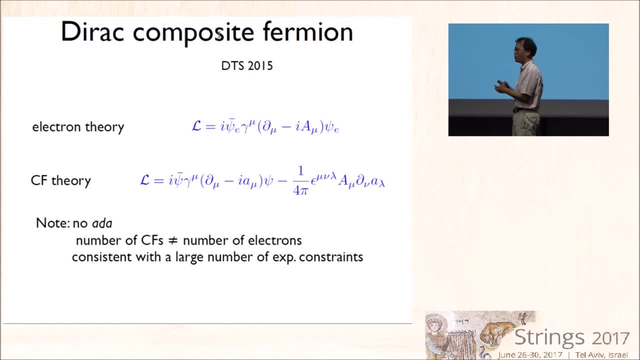 In particular this particle-hole symmetry, give a key that give a hint to how such a theory can be written down. For example, a small ADA would not exhibit any discrete symmetry that can be matched to theory. The interesting thing, I think: 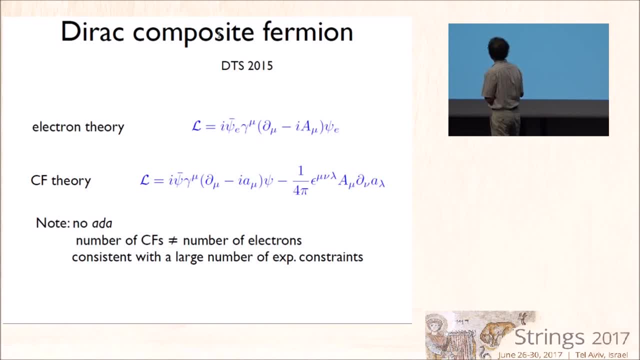 is that we know that this is, and we know from experiment, basically that this is a correct theory when the magnetic field is non-zero, And the interesting thing is that, whether the duality between these two theories can be valid also at zero magnetic field. 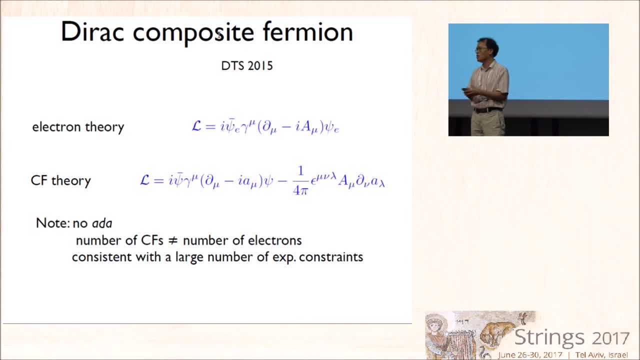 And this is, I think, a more open question, And it is basically the statement of duality. So duality is not needed per se for fractional quantum-hole effect, But I think, at least from my point of view. 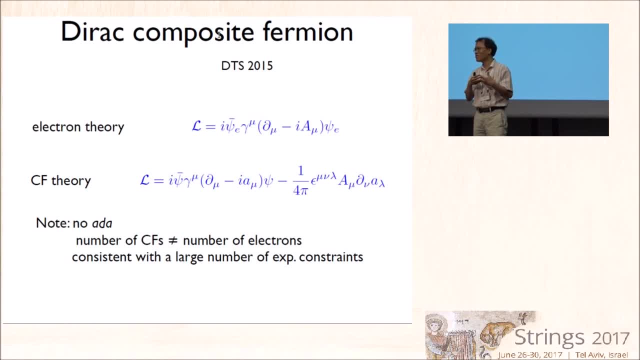 the other way, going from quantum-hole effect, one might get the hint of the duality in such a way. In the second line, Yeah, The last term doesn't seem to be correctly quantized. The last term doesn't seem to be.